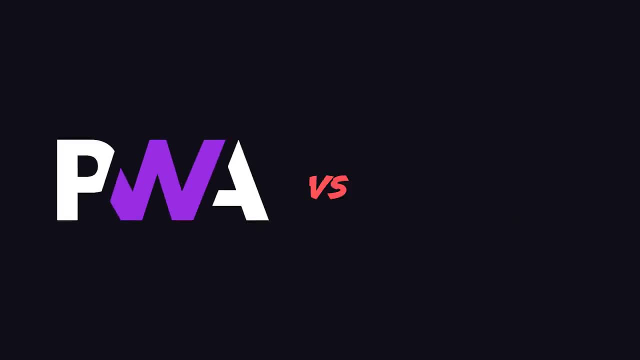 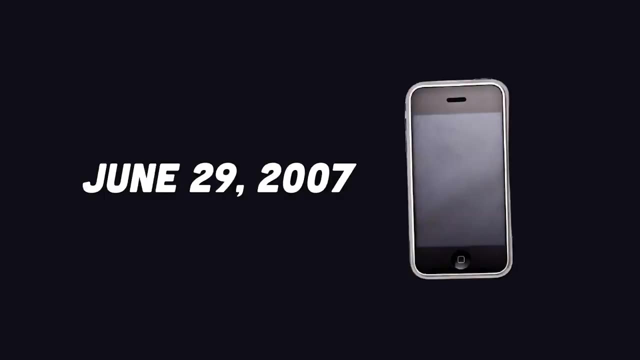 Progressive web apps. build websites that deliver an experience indistinguishable from native mobile apps. When smartphones first hit the scene back in 2008,, they brought with them all kinds of new features that weren't available on the web, like offline mode, push notifications, cameras. 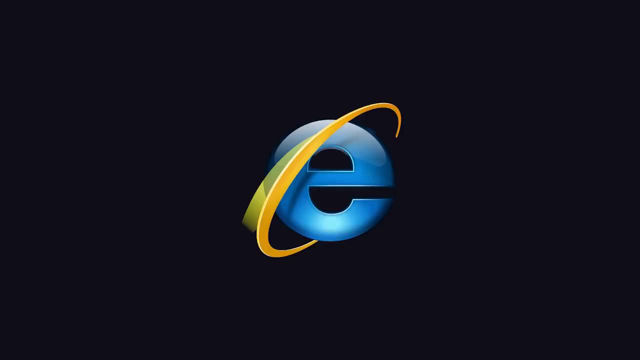 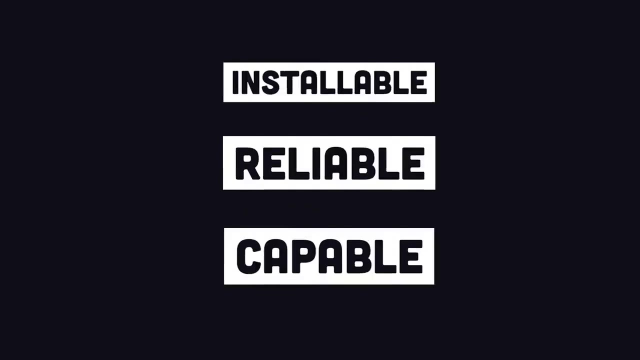 geolocation and more. Internet Explorer powered the web back then, and web developers had no way to access most in-device features. In the 2020s, though, the game has changed. The web platform has reached near-feature parity with native apps. Notice how the Twitter PWA can be installed just 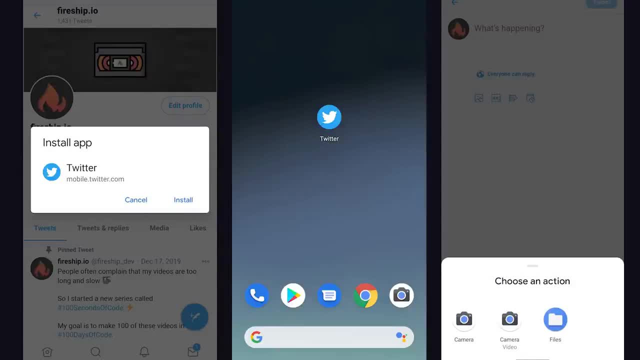 like a native app. It works without a connection, it can interact with a device camera and receive push notifications And, on top of that, the web offers much better distribution than app stores and doesn't take a 30% cut of your revenue. Not to mention, your app will work on iOS. 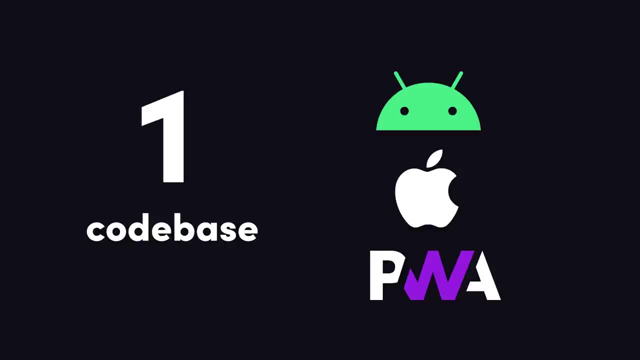 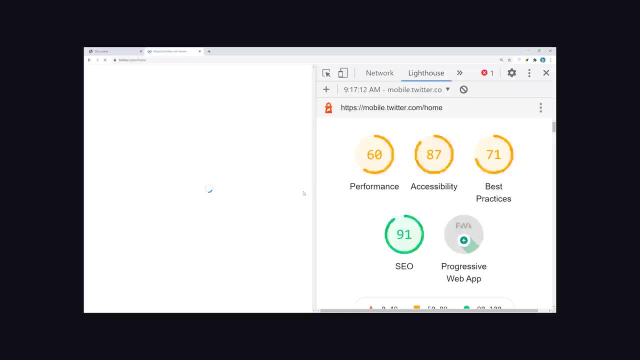 Android and the web from a single codebase. If you own a website, turning it into a progressive web app is easier than you might think. First, open up the Lighthouse tool in Chrome, DevTools- to run an audit on your site. It'll tell. 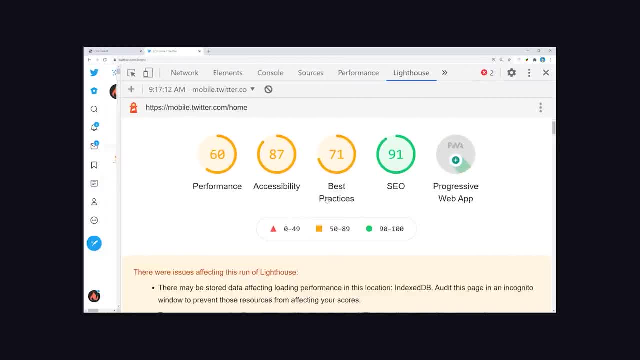 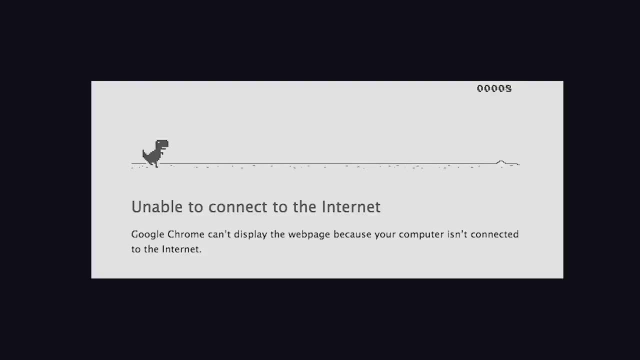 you how well your site performs and what needs to change to qualify as a PWA, At a bare minimum, the site will show you how well your site performs and what needs to change to qualify as a PWA. Most sites already check this box. The more difficult requirement is making the app work. 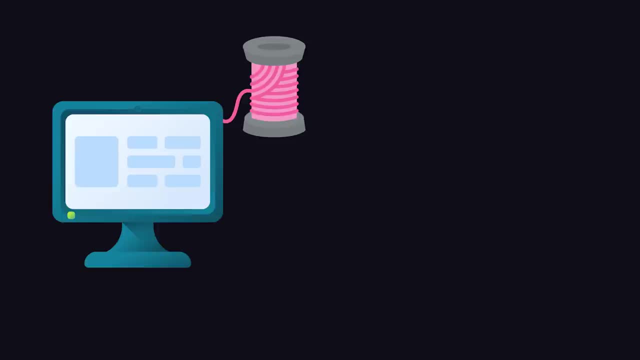 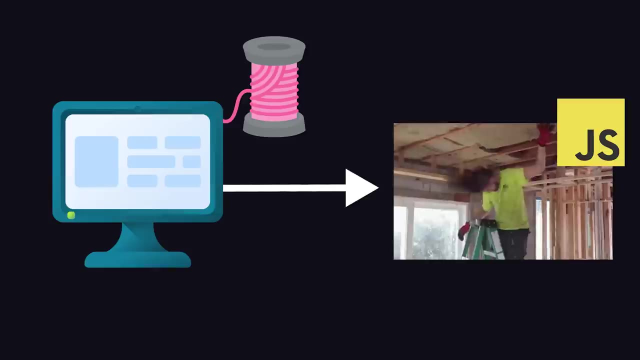 offline. Normally, a website runs on a single thread while the tab is open. However, modern websites can now register a service worker, which is just a script that runs in the background. It can perform caching, background sync and listen to push notifications, among other things. 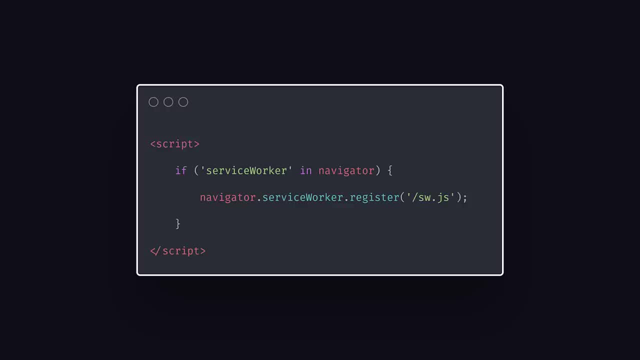 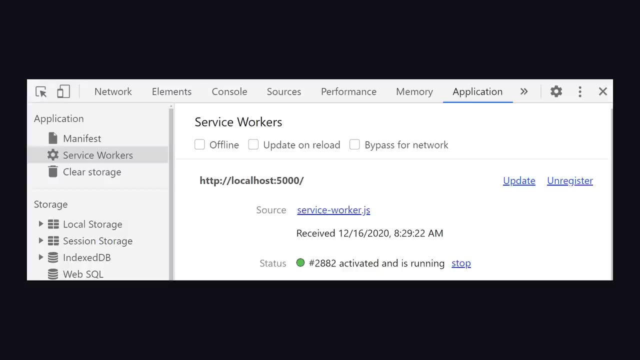 The implementation is actually very simple. We just check if the browser supports this feature. then register a JavaScript file as the worker. Once registered, you'll find it activated and the application tab in Chrome DevTools. From there you can write your own code in. 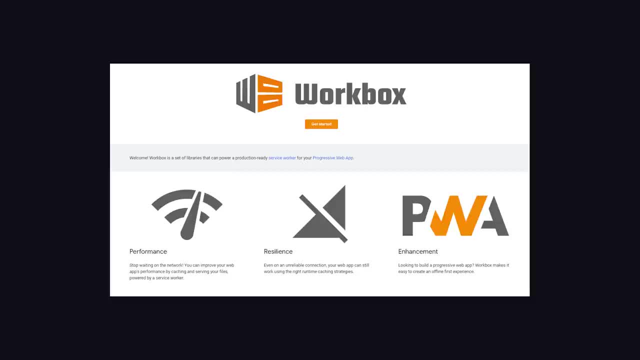 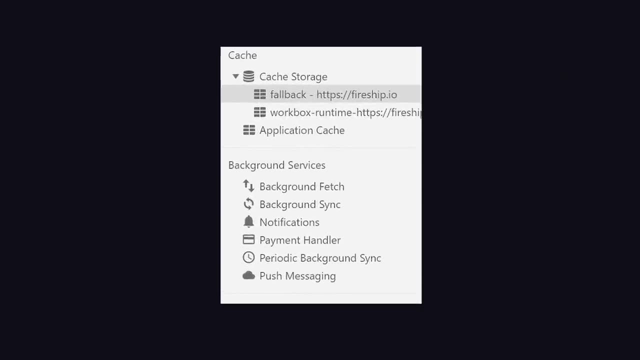 the worker file or use a library like Workbox to do everything for you. Most importantly, you'll want to cache the URLs in your app so they can be viewed offline. You can inspect the cache and other background services here in the application tab. 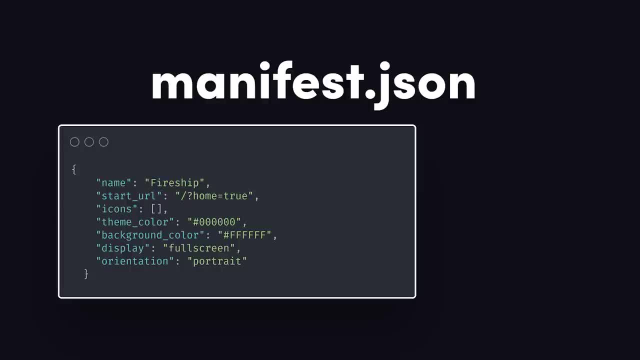 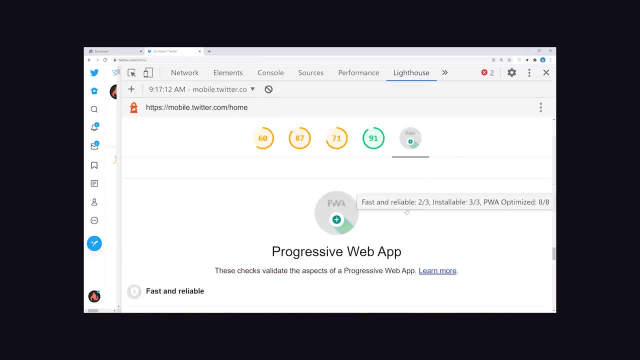 The final step is to create a manifestjson file which contains icons and other metadata about the app. Once the requirements have been met, you'll unlock the PWA Achievement in Lighthouse, at which point your app can be installed on most native devices and can even be listed on the. 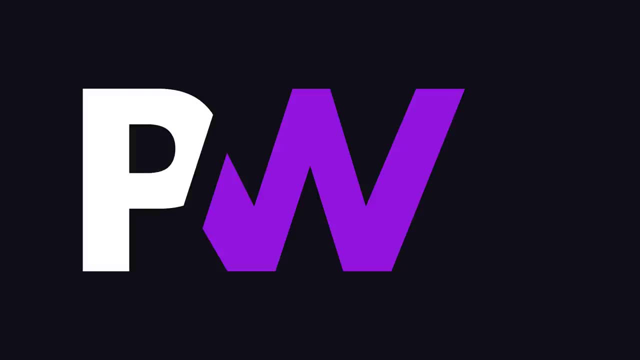 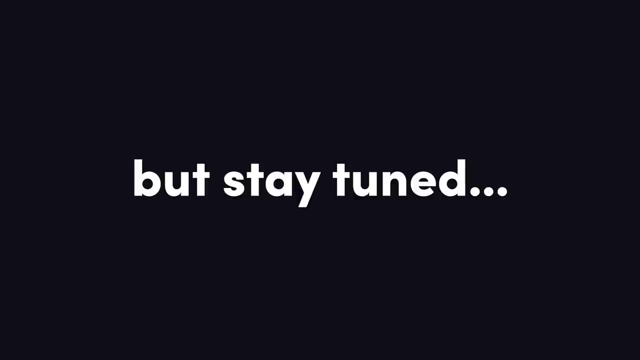 Google Play or the Microsoft Store. This has been Progressive Web Apps in 100 Seconds. If you want to learn more, hang out for a minute while we go beyond 100 seconds to learn a bunch of cool things that you'll definitely want to know about PWAs. First of all, make sure to like and 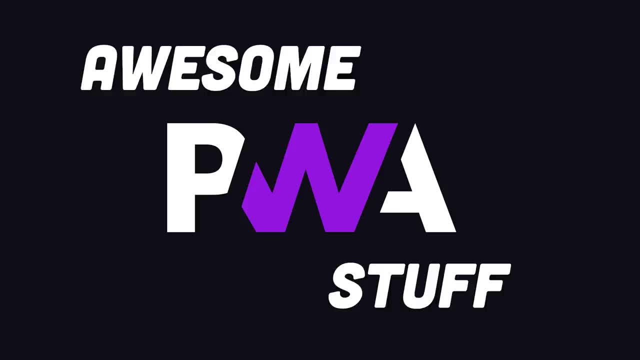 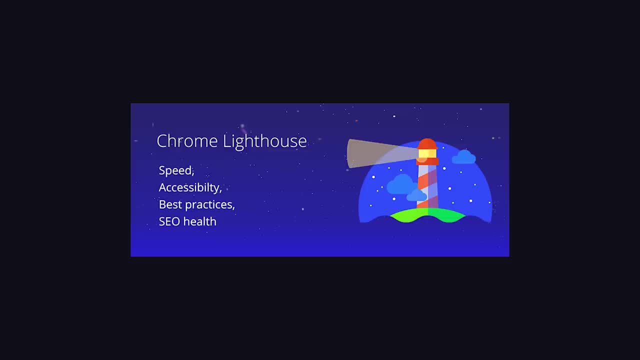 subscribe, because it really helps out these short videos. What I want to do now is just rattle off a bunch of cool things you should know about when it comes to PWAs. First, you'll definitely want to get familiar with the Chrome Lighthouse tool. It analyzes performance, accessibility, SEO. 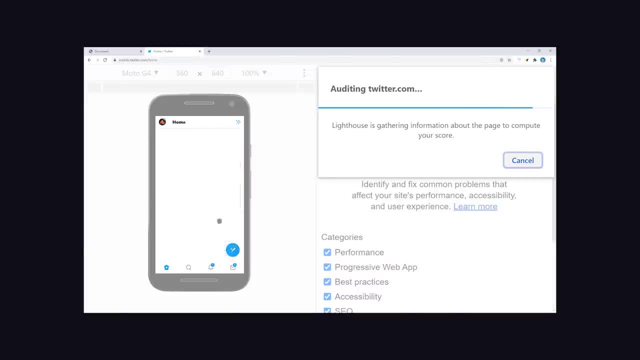 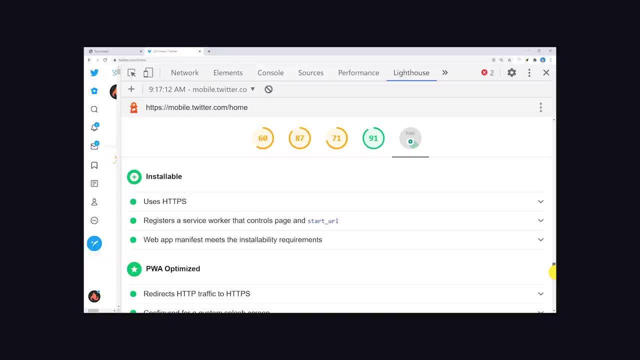 and determines whether or not your app is installable as a PWA. You can run this tool on any site you want and should be available under the Lighthouse tab in Chrome DevTools. Even if you're not building a PWA, it can be useful to run an. 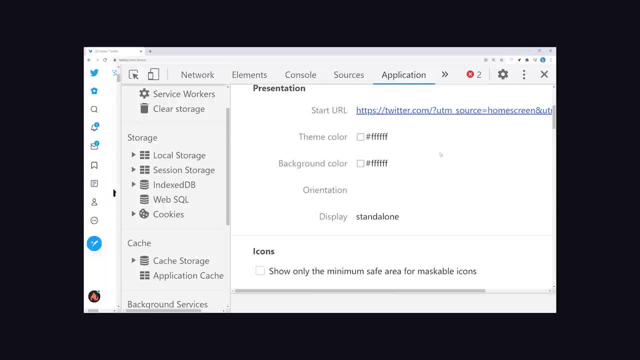 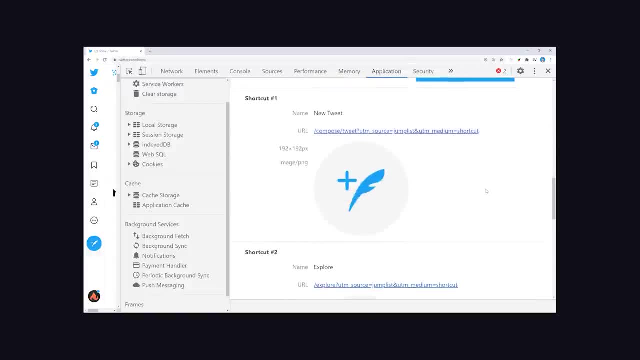 audit on your site. And, while we're here, you'll also want to know about the Application tab, which allows you to analyze and debug information related to your app. Every PWA has a manifest file which defines metadata about the app, and you can view that here, such as the app name and icons. 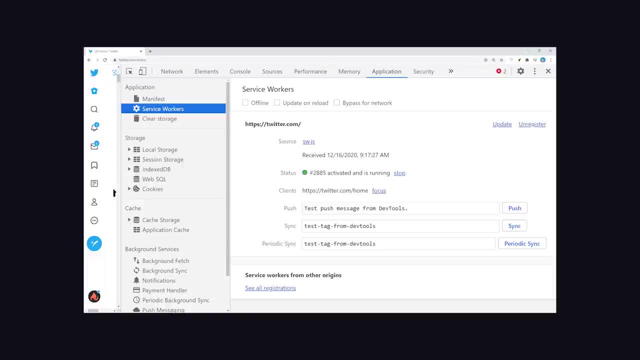 But more importantly, it tells you whether or not a service worker is up and running. You can also manually trigger events here to test things like push notifications and background sync. Your service worker will likely cache pages and you can view the cache from this tab as well. 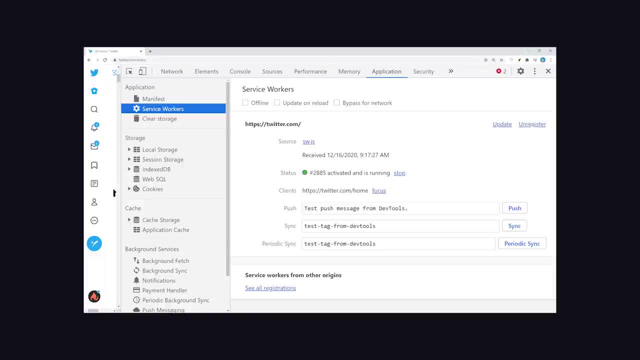 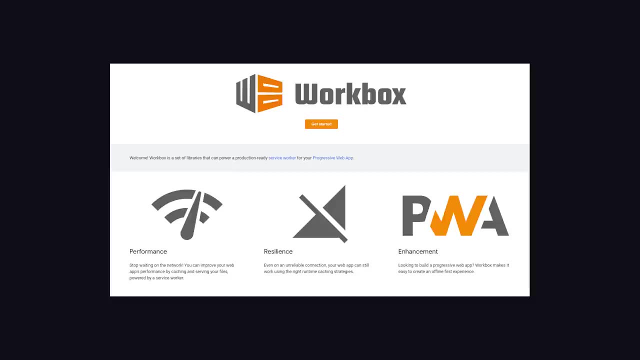 Now, when you hear me talk about service workers and caching, that may sound like a lot of code that you have to write, but that's actually not the case. Most of these jobs fall into very common use cases and can be implemented with minimal code if you use a library like Workbox As the 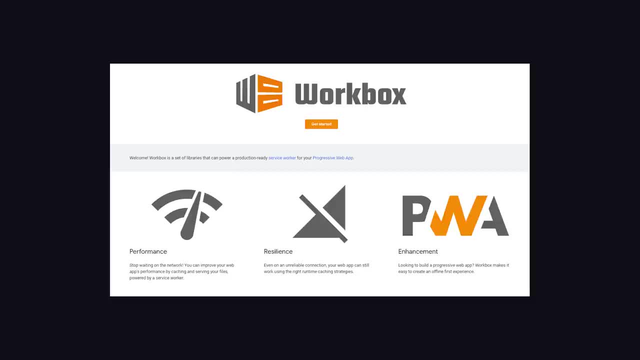 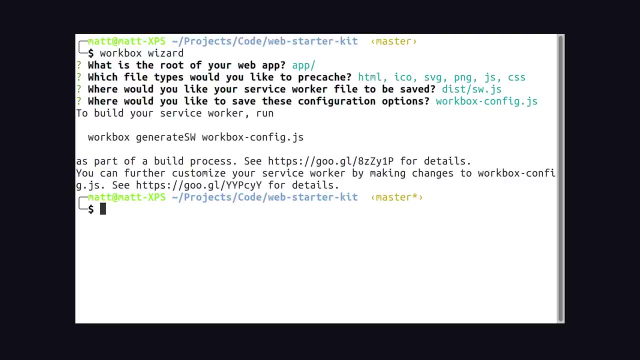 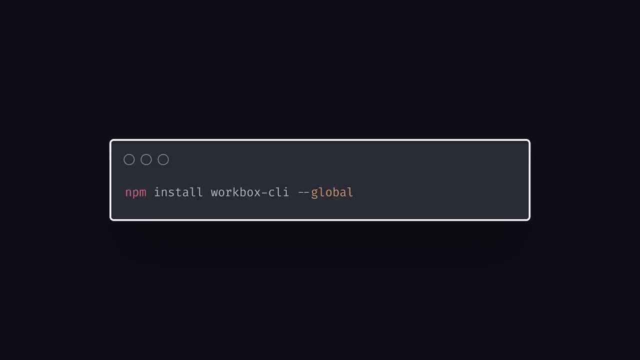 name implies, it's a collection of different libraries to help you build PWAs quickly and reliably, And it even has a CLI tool to automatically generate the files and assets that you need. If you're using a front-end framework like React or Angular, you can install it as an NPM package or you can import it directly into. 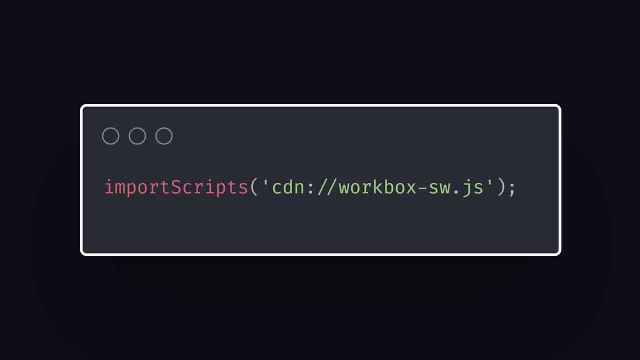 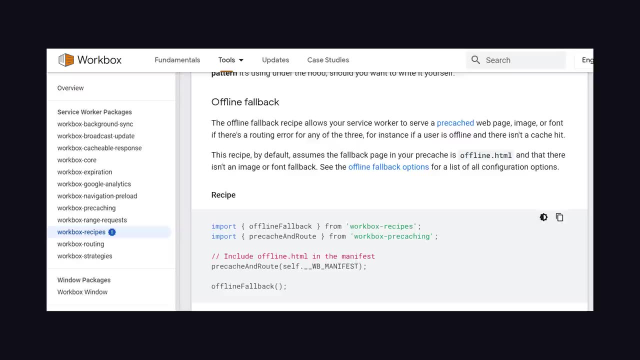 your service worker over a CDN using the import scripts function. But an awesome new feature in Workbox is recipes. It allows you to implement features very quickly, often with just a single line of code. Want to add offline fallback to your app? It's just a single function call. 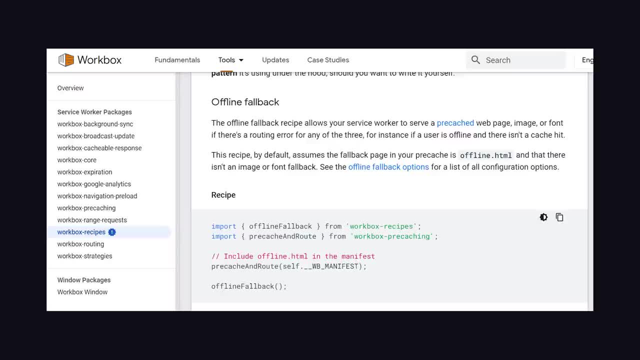 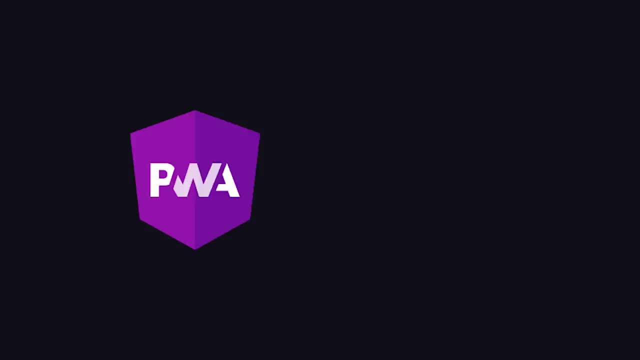 And the same goes for an image cache, Google Fonts cache and many others. Workbox is awesome. there are other libraries out there as well. If you use a framework like Angular, it has a service worker module built into it, And when you use the Create React App tool, 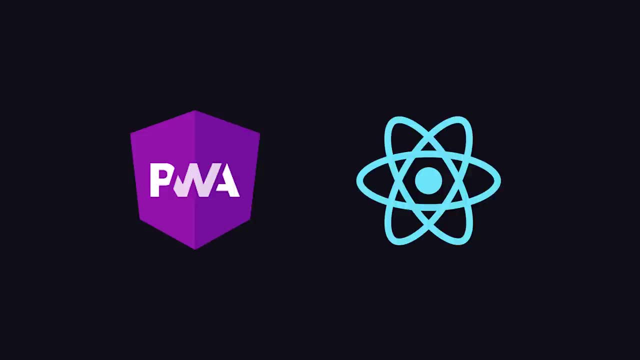 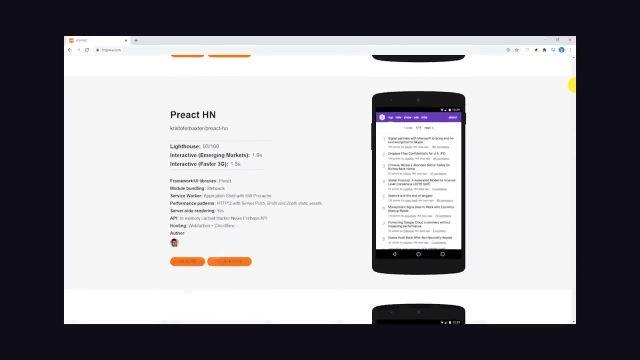 it automatically generates a service worker for you. And speaking of frameworks, if you want to see how PWAs are implemented in a variety of different frameworks, check out the Hacker News PWA site. It's a showcase of different framework implementations and how well they perform compared to each other. If you're learning to code, a great project is. 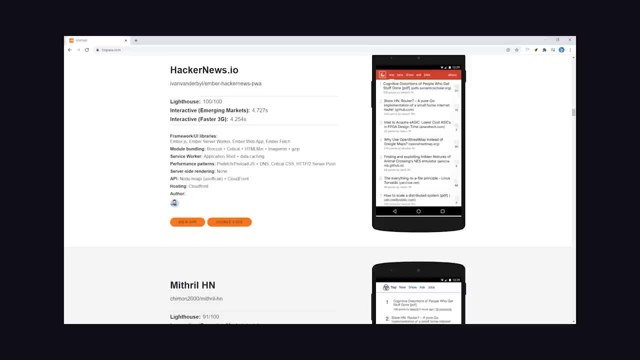 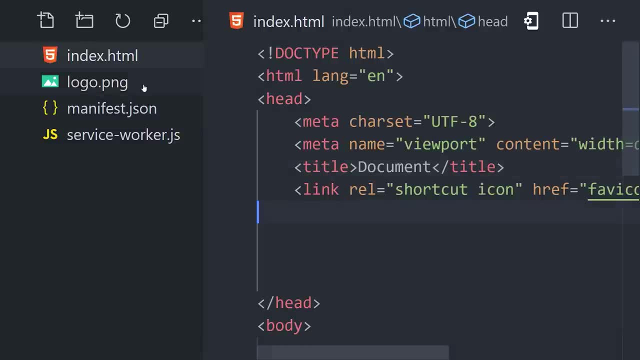 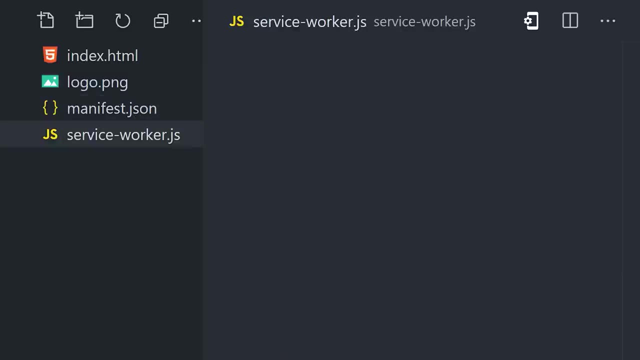 implementing your own version of a Hacker News PWA. Or if you want to start with something easier, let's go ahead and build a PWA. right now. We only need four files: an index HTML for our main web page, a logo, a manifestjson to describe our app and then a serviceworkerjs file. 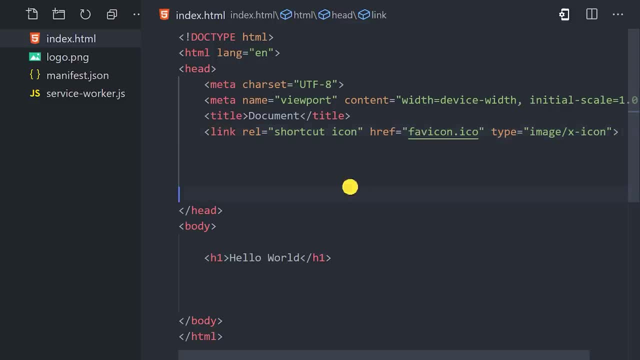 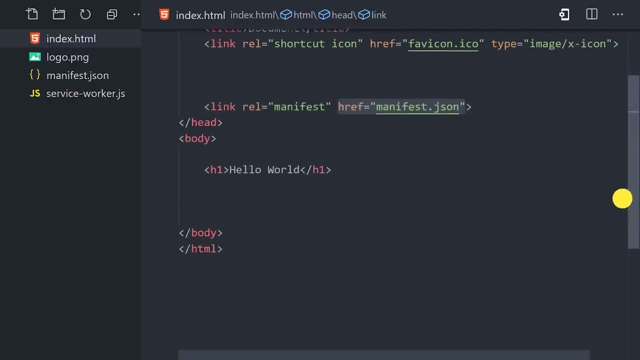 The HTML needs to reference the manifest and load the service worker. We can reference the manifest with a link tag, just like we would with a CSS file. Then we can add a script above the closing body tag And if the service worker is supported in this browser or in its navigator, then we'll go. 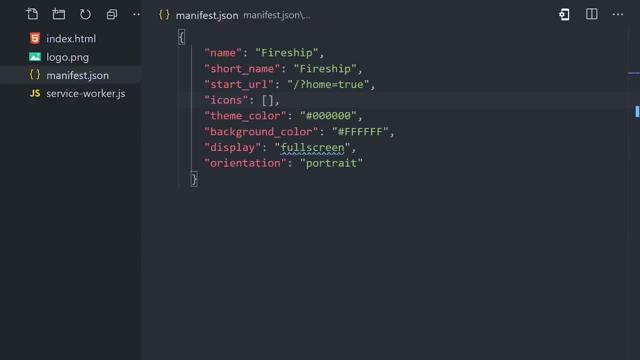 ahead and register our service worker file. Now, if we open up the manifestjson file, we can add some information about our app, which is mostly self-explanatory. But notice this icons array. It's looking for icons or images of different sizes. that can be. 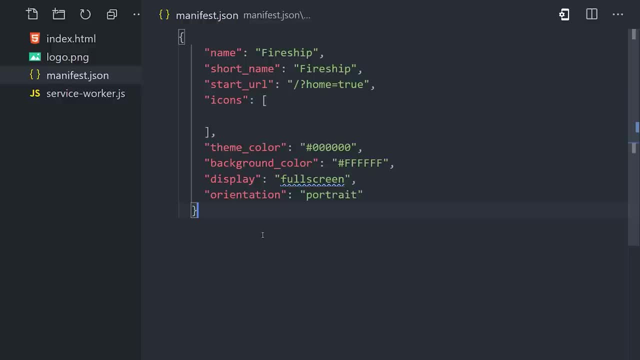 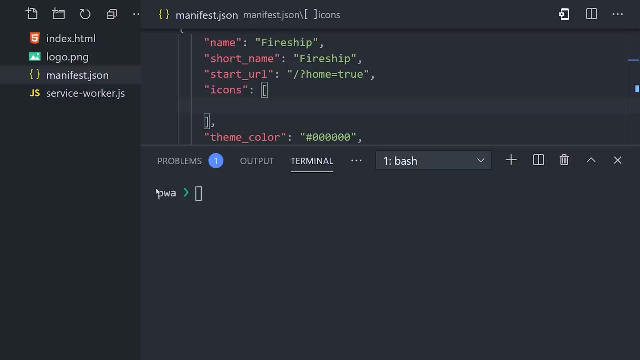 used as the home screen icon for our app. We could create all of them manually, but that would take forever. A better option is to use the PWA asset generator. We'll go ahead and run npx PWA asset generator, then point it to the logo file in our project and tell it to. 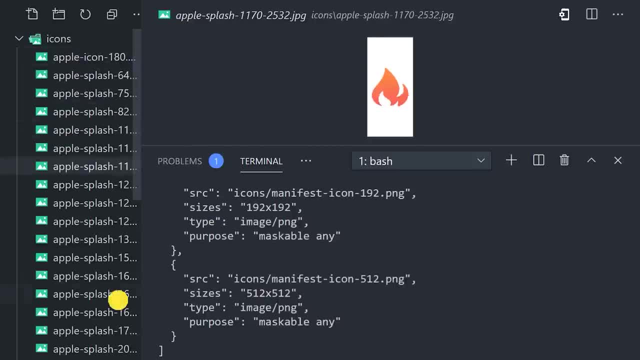 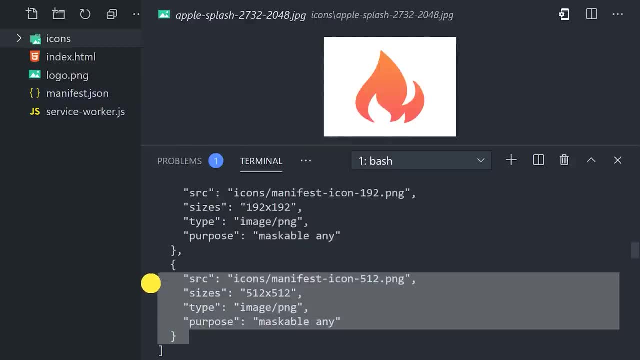 output the results in the icons directory. That creates a bunch of images for us in no time, And if you look at the terminal output, it'll even give you the JSON that you need to paste into your manifestjson file. Now we just need to write a little bit of code in our serviceworkerjs file. 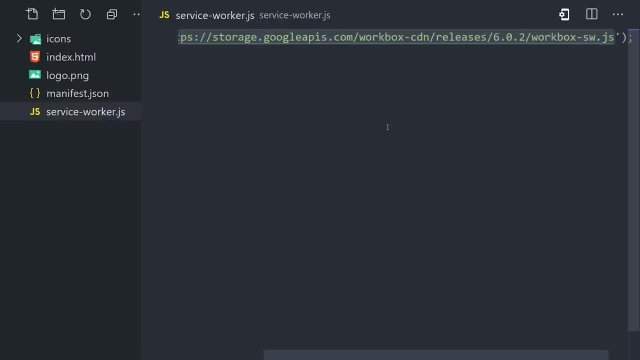 to enable caching, We'll import Workbox from a CDN by adding a link to the file inside of this import scripts function. That'll give us access to Workbox. Then we can use the routing module to register a route that matches all the image files in our project. 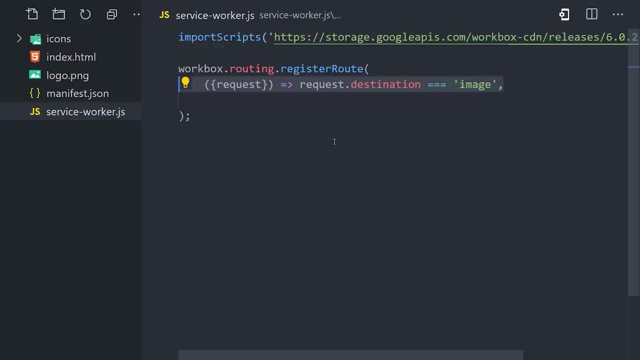 Once we've matched all the files, we need to decide on a caching strategy. In this case, we'll use cache first, which means the PWA will attempt to read from the cache instead of going over the network, if there's something available in the cache.